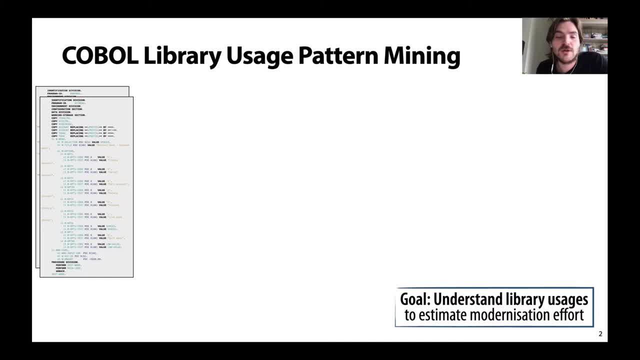 in the banking industry and really everywhere you look. So a lot of these code bases are very large and very old and every once in a while they might have to be migrated to a new platform. And if these code bases use libraries, the libraries will also have to be migrated to that. 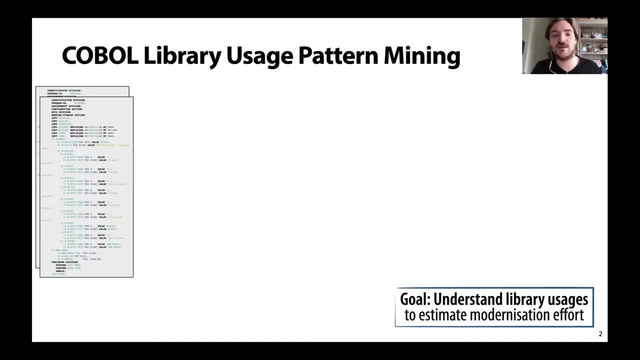 new platform. But in some cases that's infeasible because of legal issues, because of technical issues, So they have to be re-implemented Now. you're not going to be re-implementing a library without properly gauging how much effort it would take, And to do that you really need to understand. 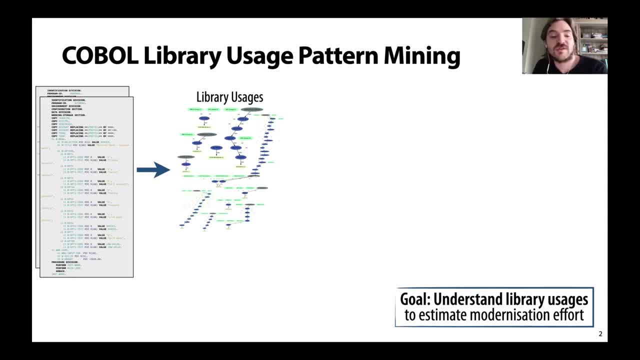 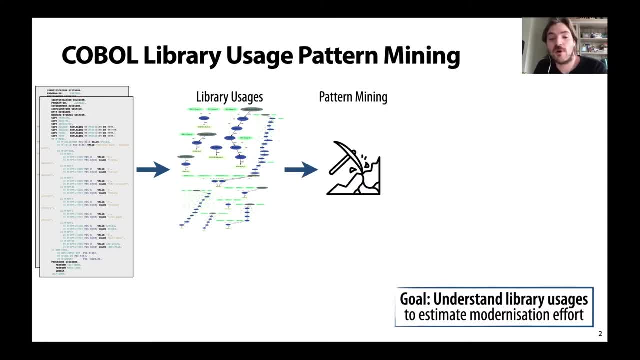 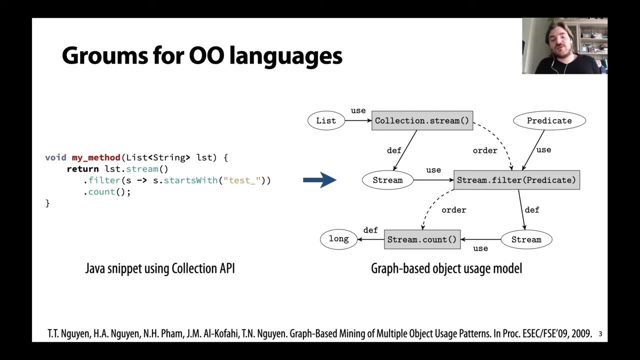 From a global code base, use some sort of pattern mining algorithm on these library usages and inspect the resulting library usage patterns to then estimate the amount of effort that it would take to modernize these. So there's also already been a lot of research in library. 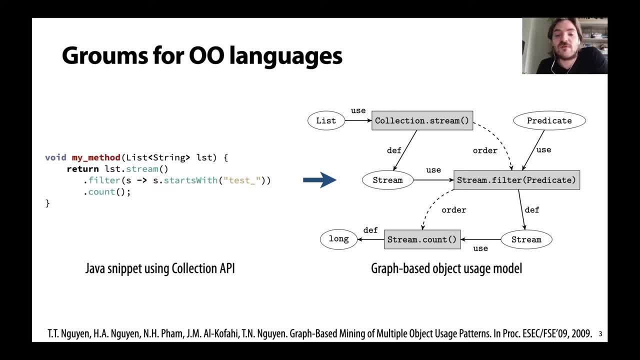 usage pattern mining, especially for object-oriented languages. For legacy languages not so much So. for example, you have GrooMiner, which uses grooms or graph-based object usage models for Java methods, And these grooms contain some library calls and the control flow between 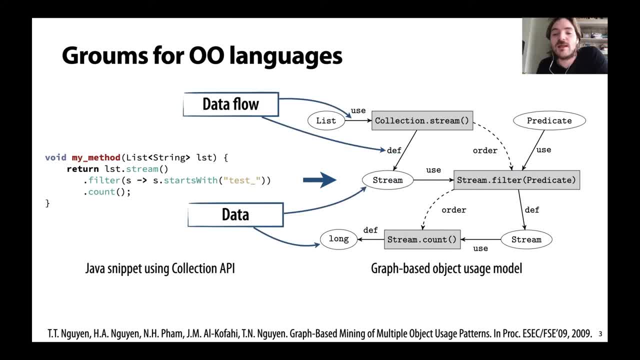 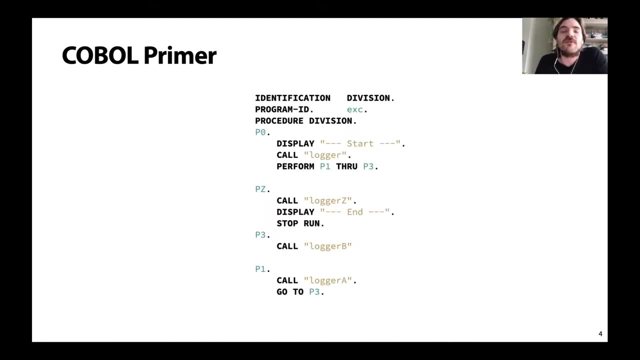 these library calls, These are really control flow graphs. And then there's also data and data flow edges that describe how data is used in these library usages. And then these grooms can later be mined to find patterns. And we're thinking, okay, let's apply this to COBOL, But of course, 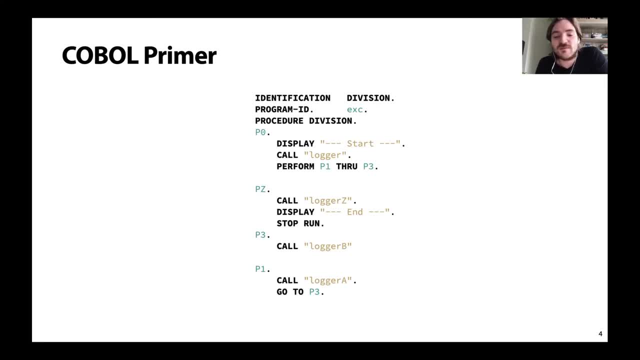 COBOL is fundamentally different from object-oriented languages. In Java you have methods. In COBOL you don't have methods. There's paragraphs, but those are just labeled sequences of statements. If you don't have methods, you don't have method calls. Instead, you have a call statement that. 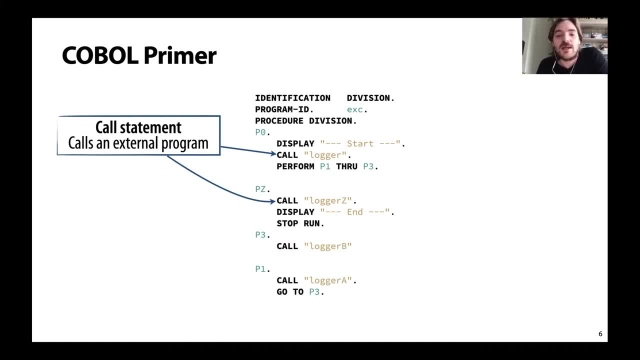 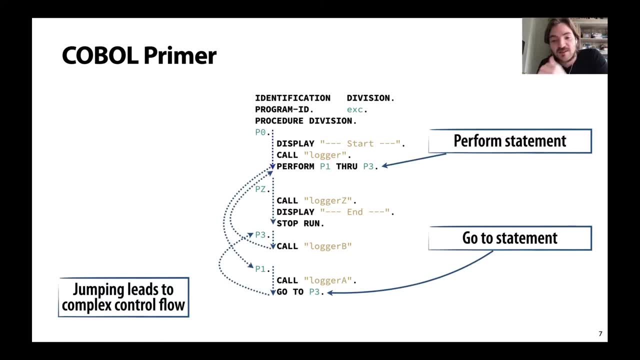 calls another program written in some other file, And well, that's very different from a method call. And, of course, because COBOL is a legacy language, you have these legacy control flow constructs such as goto and perform, And that should really send chills down everyone's spine. 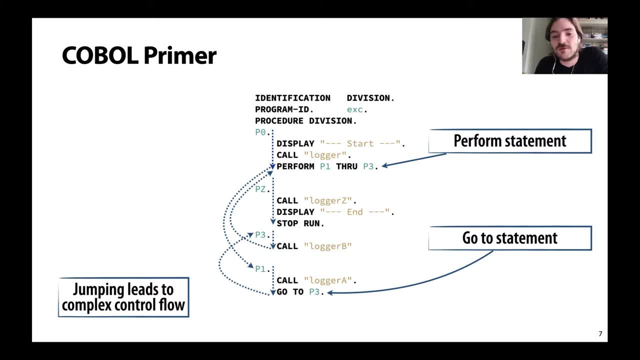 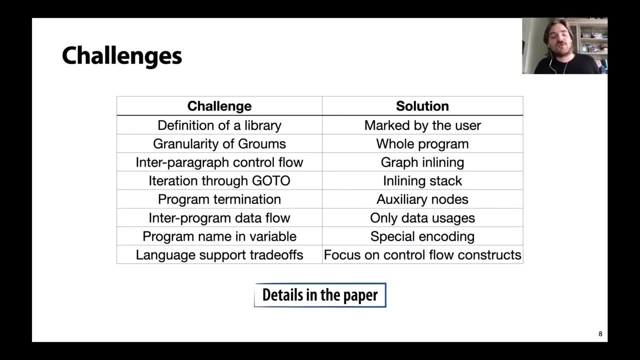 because the combination of these two leads to very complex control flow, kind of spaghetti codes as you wish, even in this very small example. So trying to extract grooms for COBOL codes, well, that poses a number of challenges, I'm. 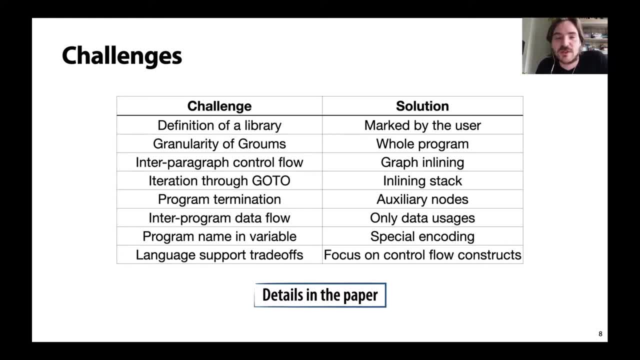 not going to go too much into detail in every one of these, into every one of these, but full details can be found in the paper for anyone who's interested. Now, for example, just the definition of what the library actually is is already quite fuzzy in COBOL, So we rely on the. 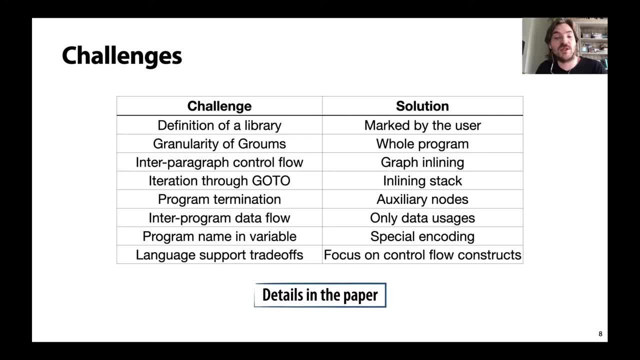 user to mark specific programs as being part of a library. Any call to these programs would then be considered a library call. Also, the granularity of grooms is well different in COBOL than it would be in OO languages, For example. in Java you can say, okay, one method is one groom, but 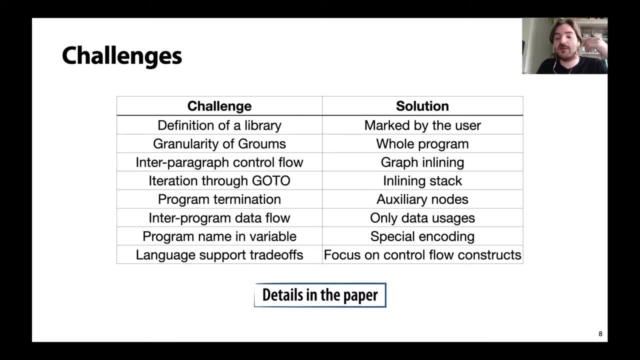 since you don't have methods, that principle obviously doesn't apply. And looking at a separate paragraph, an individual paragraph for each groom, leads to some issues with the grooms being too small. So we have to look at the whole program And then, of course, you have to look at the 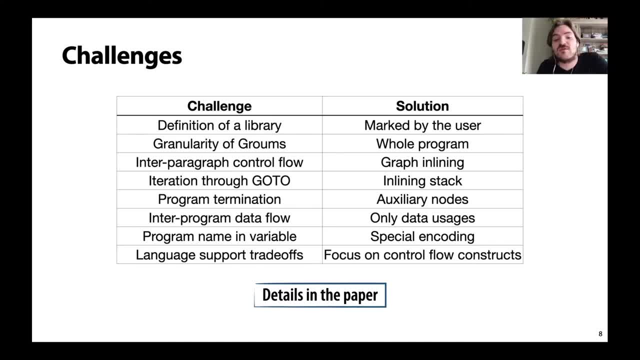 program as one single groom. Looking at the whole program leads to interparagraph control flow which needs to be accounted for. There's also the possibility of iteration through the use of gotos, whereas grooms are actually acyclic. so that has to be handled And we also need to make 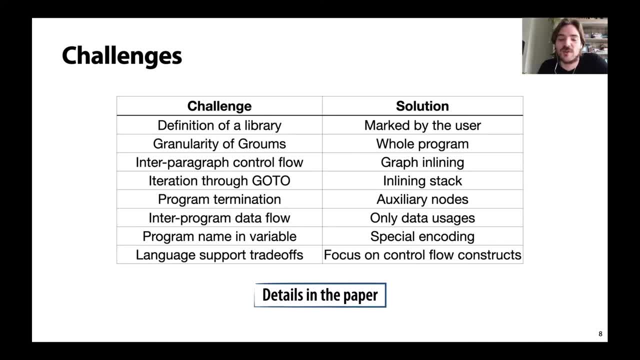 sure that we understand how the program terminates and where the program terminates, because otherwise our grooms won't really be that representative. There's also a range of other issues which I'm not going to describe here, though, Like I said, single paragraphs are a bit too small for a single groom in COBOL. 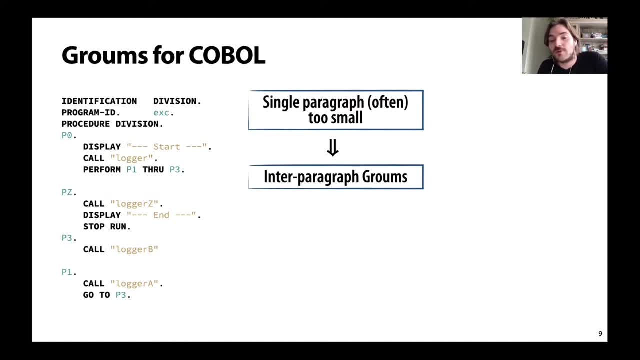 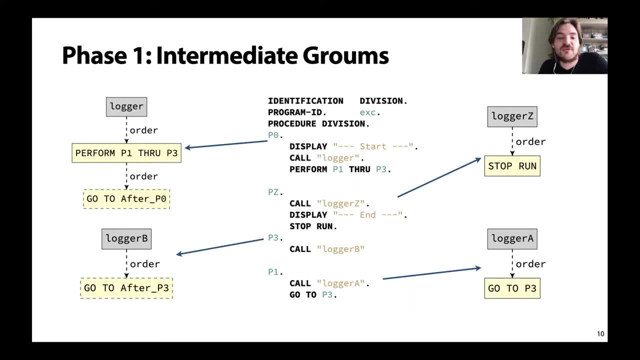 So instead we're looking at interparagraph grooms, more specifically whole program grooms. so we have to account for interparagraph control flow, which we do via graph inlining. Now our extraction process is two-phased. In the first phase we create intermediate grooms for 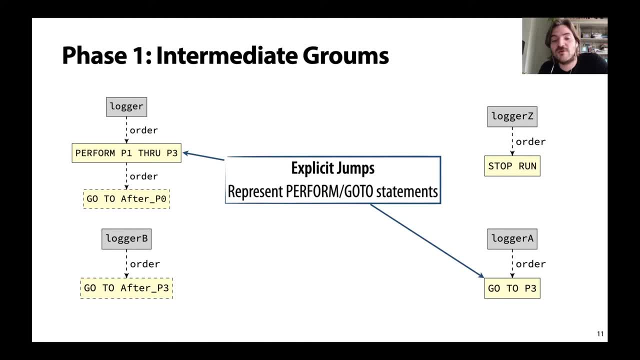 each paragraph individually. These contain some auxiliary nodes, such as the explicit jumps that happen in the source code itself. like these perform and go to statements, as well as the names that happen at the end of a paragraph, that may go to the next paragraph or some other point. 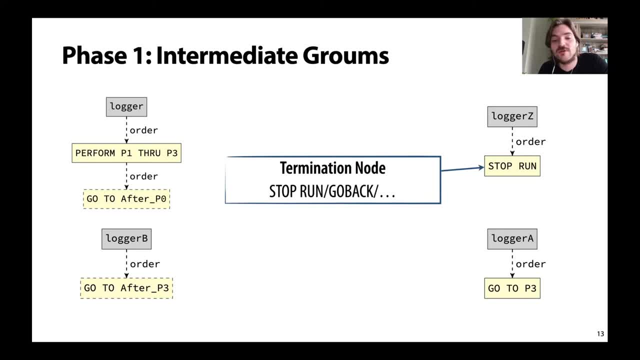 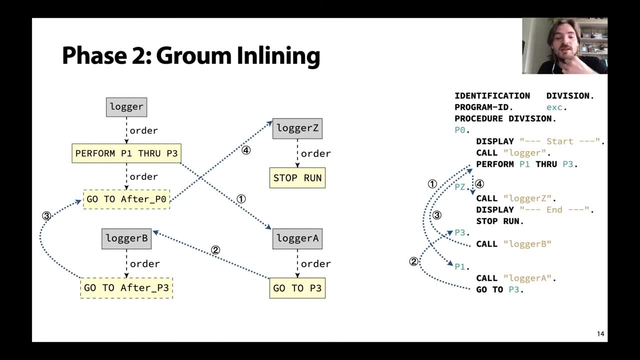 in the program. And then there's also the termination nodes that will mark when a program stops and subsequently also the groom should stop. And then all of these intermediate grooms can be linked together in phase 2 in the same way that the program would jump between. 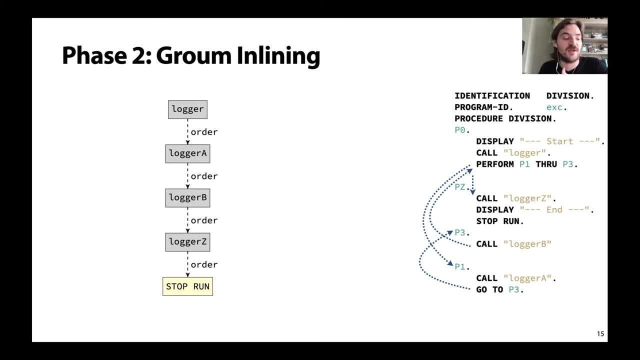 these paragraphs at runtime and then, when they're inline, you get this very nice and succinct representation of which calls are made, in which order. conditional. in the example, there would have been a branch in this graph as well, but that is not the case right now, So we can extract these grooms. but the main. 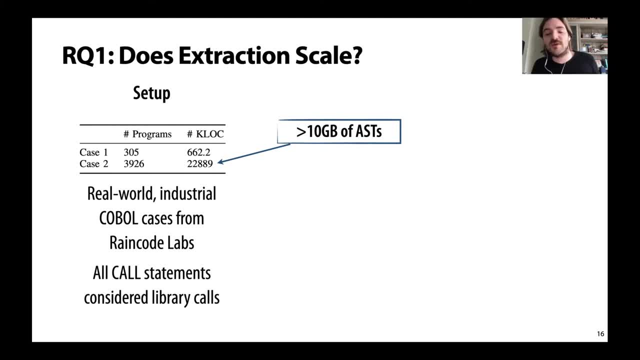 question is: can extraction actually scale to very large global code bases, because a lot of these code bases have millions upon millions of lines of code. To evaluate this, we took two real-world industrial global code bases that were provided by raincoat labs. The second of these two cases has nearly 23 million. 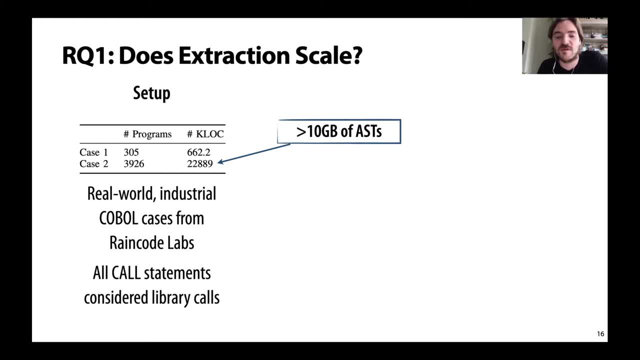 lines of code. It's represented by well over 10 gigabytes worth of ASTs, so that's a really good case to actually gauge how performant or how efficient this extraction actually is. So if we extract grooms from both of these cases, we get a runtime of about 17 minutes for the second case, which 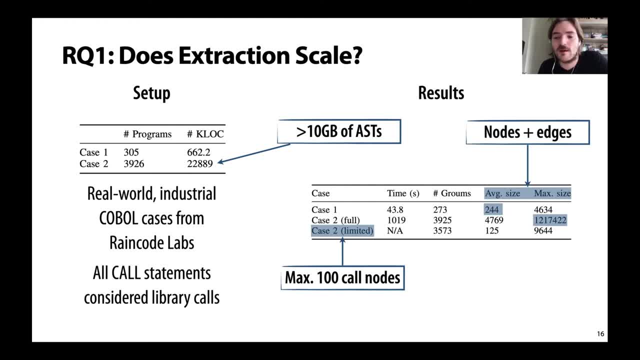 is really commendable given the size of the code base. But what we also find is that our grooms are well, fairly large. They're in general larger than object-oriented grooms, which is to be expected because they're whole program instead of single method. But also some of these grooms are very, very 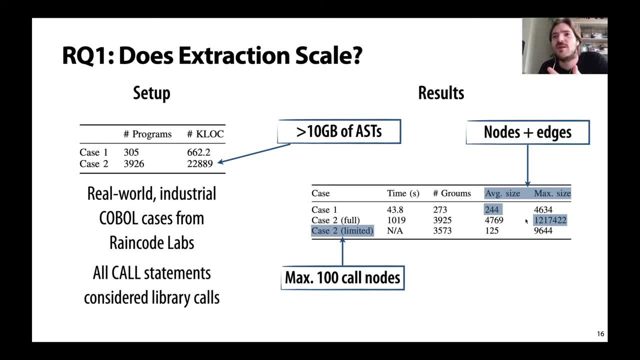 large, with more than a million edges, which has to do with a lot of the spaghetti code and a lot of the branching, and we already expect that these grooms probably won't be able to be mined by any mining algorithm right now. So we created a third corpus, the limited case 2 corpus, where we remove 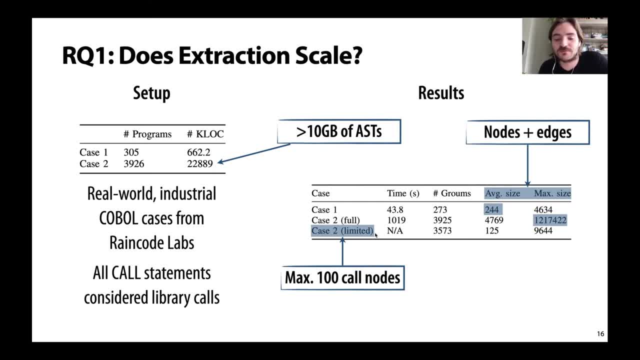 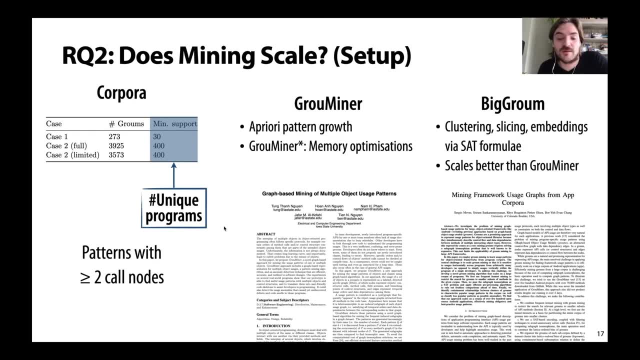 any graph that has more than 100 call nodes from consideration. Speaking of mining, we're also looking into whether mining actually scales and whether mining actually can be done in reasonable time. for these cases, We took the three corpora from the previous slide, and then we also took two. 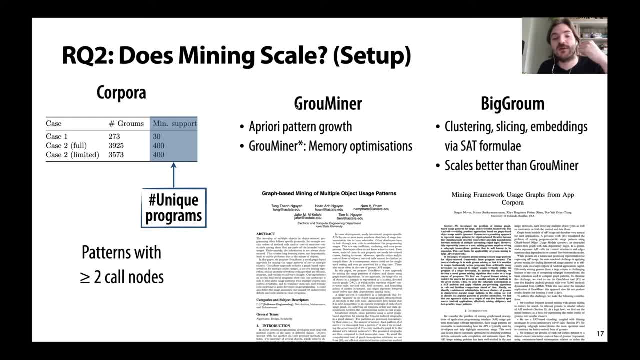 different approaches. on mining. We have the original grubminer approach, which is an a priori pattern growth algorithm. We made some memory optimizations to make it handle very large graphs, but the core algorithm remains the same. And on the other hand we have room, which does some optimizations. it uses clustering to partition the grooms it uses. 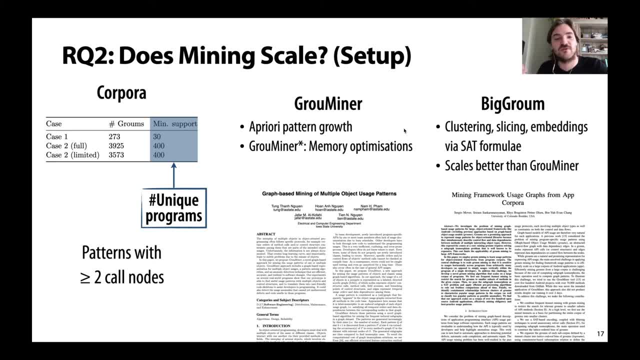 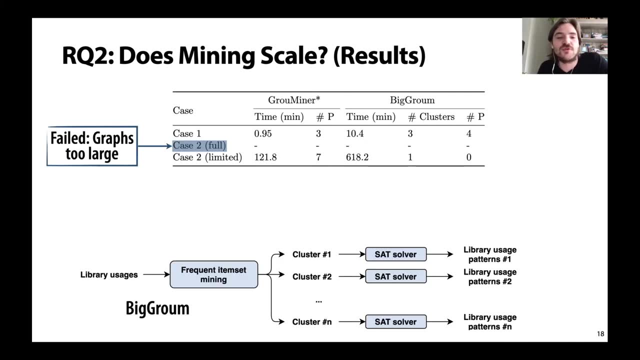 slicing to shrink the grooms and then uses set solvers and set formulae to find the frequent patterns, and it has been shown to scale better than groom miner, at least for java code. now we're wondering whether that will apply to cobble grooms as well and when we run these things, unfortunately, 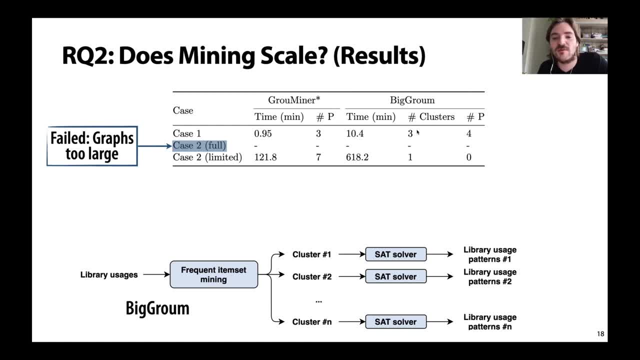 we find the exact opposite case. it doesn't really scale well for our cobble grooms. but first, first and foremost, our full case, two corpus. neither of the two approaches actually mine this properly. groom miner runs out of memory even though there was 32 gigabytes of heap space assigned to it. 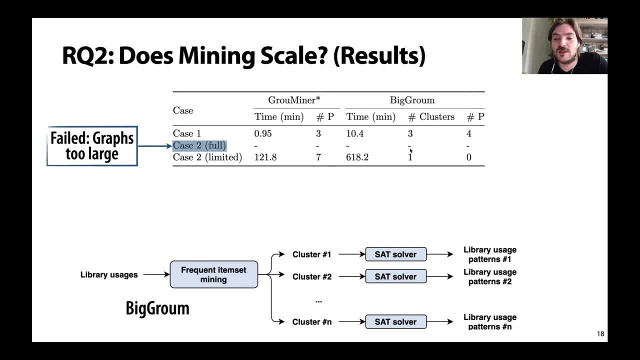 big room runs into overflow issues with the formulae, so it can also not actually mine any of these graphs. some of these graphs are just too large for either of the two approaches. but for the limited case two corpus, we find that gru miner takes about two hours producing seven patterns. 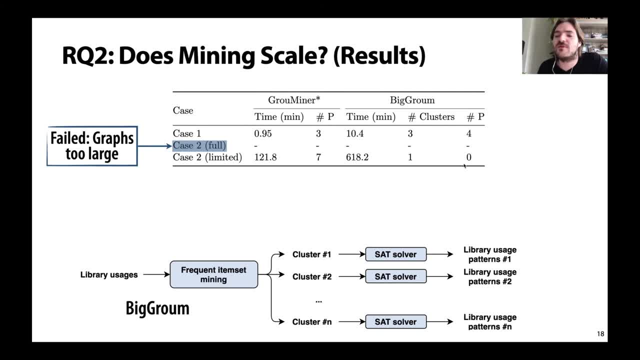 big room, on the other hand, takes more than 10 hours and doesn't produce any pattern whatsoever, which is really surprising, because we expected it to scale better than gru miner and evidently it doesn't. so we looked into why this actually happens and if you look at the architecture of big room, it actually takes all of 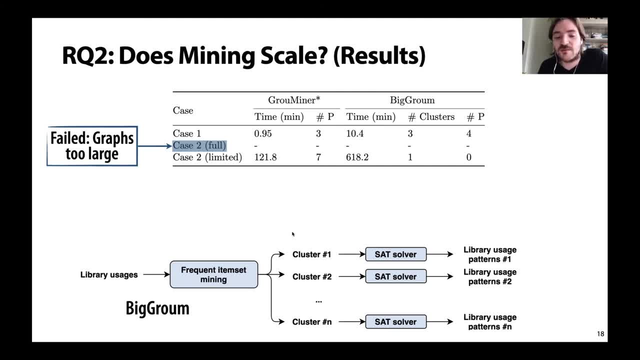 these library usages, uses frequent items of mining to cluster them into separate clusters based on the call labels, based on the methods or the programs that are called in these grooms. so one is called the same programs and then these are further sliced and fed into a set solver to find 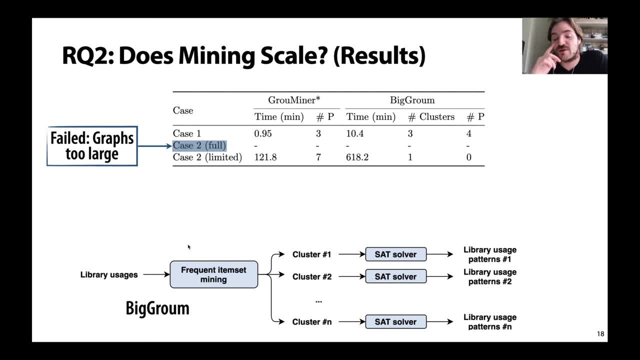 the frequent patterns for java. this works because you have a lot of different apis. you have a large alphabet of different skull labels, so we can get a large number of clusters that don't contain that many graphs each, and these graphs can then also be further sliced and fed into the set solver. 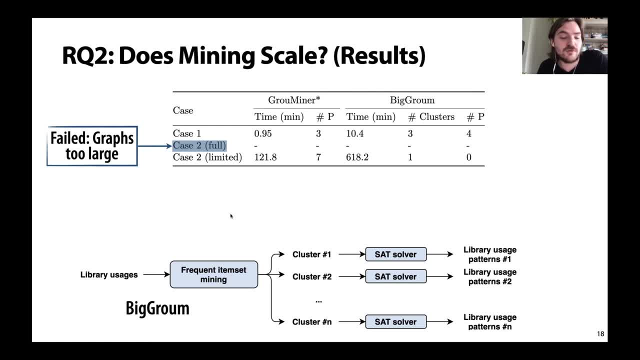 whereas in our case we have, for example, for the limited case two corpus, we have 3500 programs, but in unique call labels. so we only get one cluster after the clustering. this cluster contains all of the grooms. they cannot be further sliced. they're fed into the sat solver as is. these calls are very 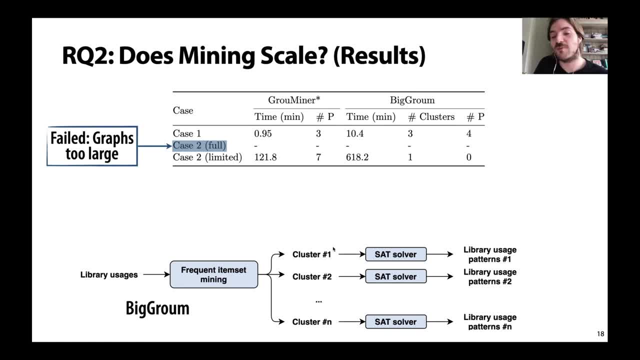 expensive and it doesn't find any pattern whatsoever. so the bottom line is that big room actually makes some assumptions about the nature of these grooms. that doesn't hold for global grooms. so, to conclude, i've presented an approach of mining library usage patterns in global codes. 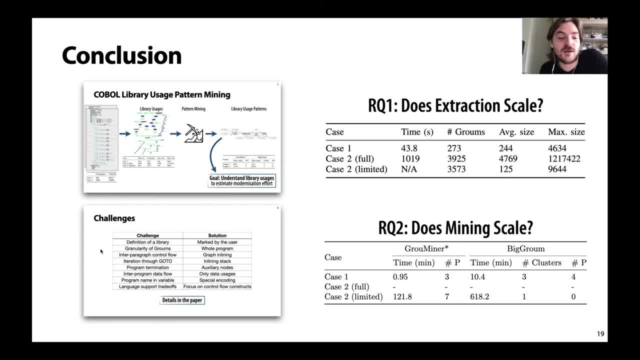 i've talked a bit about the challenges that we ran into, mainly interparagraph control flow, and how we overcome these challenges. i've shown you that we're pretty confident that our extraction will scale to very large global code bases and that mining can be done in reasonable time given. 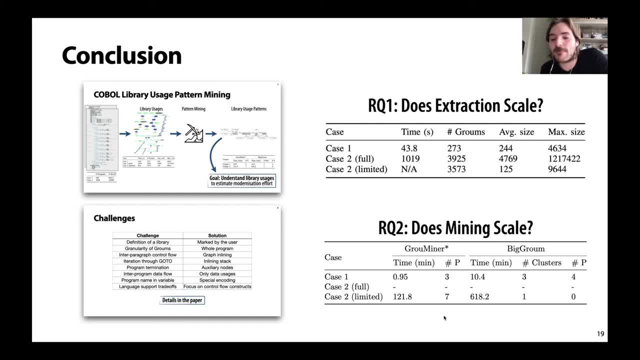 that you use an a priori pattern growth algorithm, whereas if you use big room, which does scale better for java, that's actually not the case. it doesn't scale better for global. with that i end this presentation. thank you all for listening and if you have any further questions, i'm sure. 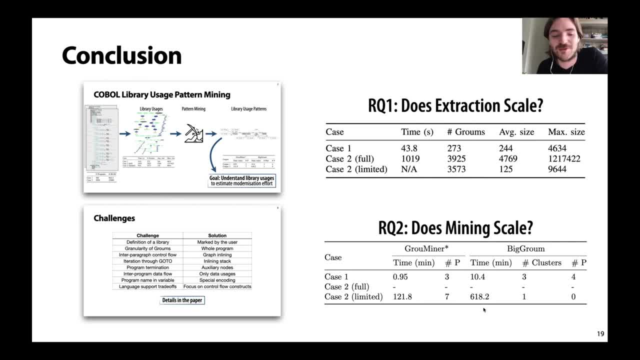 reuben in the future will be more than happy to answer them. thank you. 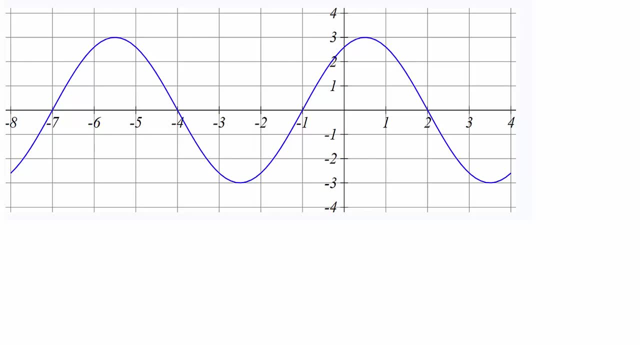 Okay, on this graph we're going to find the equation of this sinusoid, and so we're going to find out different pieces of it. The first thing we're going to do is mark the baseline. It goes through the middle, it's the line that it's oscillating about and that's going to be at y equals zero, so there's not a vertical shift. The next thing I'm going to do is determine the amplitude, and I see from the baseline I go as high and as low as three away, and so the amplitude is going to be at zero.